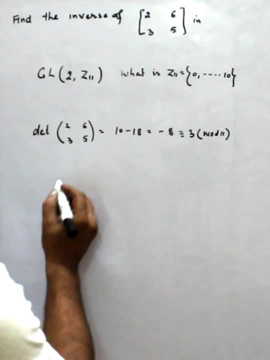 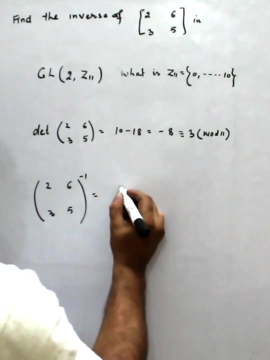 will find that joint That is the inverse. or we can say I write 2,, 6,, 3, 5, inverse of this matrix is equal to 1 by determinant, that is, 1 by 3 into the cofactor of this. 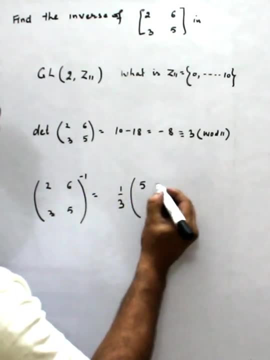 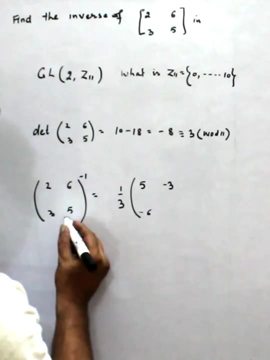 matrix and this number, 2, is 5.. And the cofactor of this matrix X is equal to 1 by determinant, that is 1 by嘛1 sushi3. prejudice of 6 is minus 3 and this is minus 6, and cofactor of 2 is 5 is 2, and here is the. 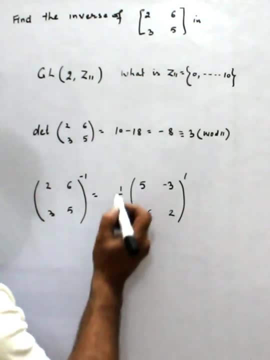 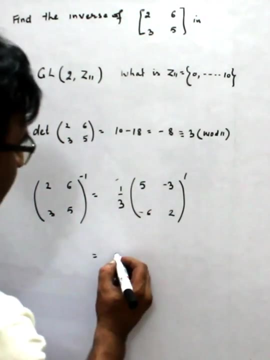 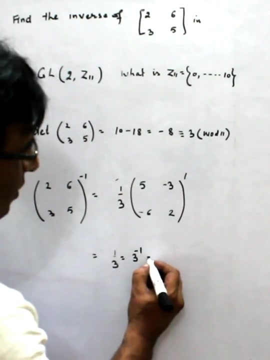 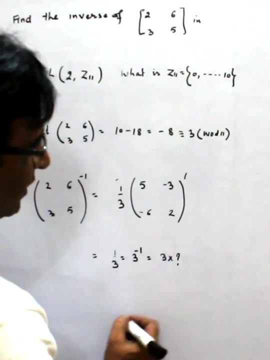 transpose. so this become first this: 1 by 3, also not there. so first we find what is the 1 by 3. 1 by 3 I can write equal to 3 inverse, that means the multiplicative inverse. actually. so with what I multiplied with 3 so that I get. 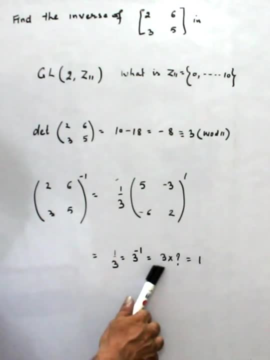 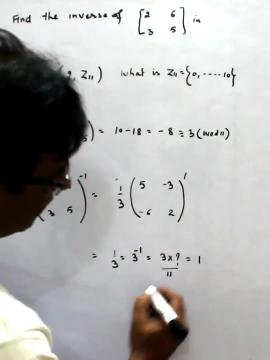 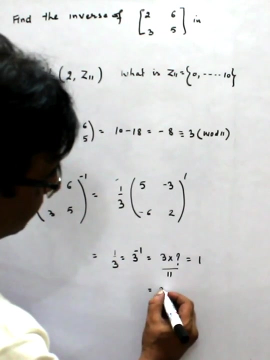 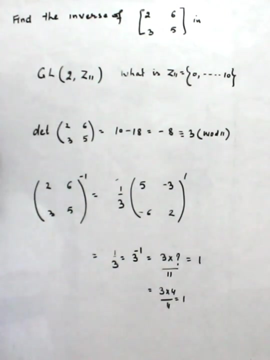 the remainder 1, the. simply you can see that if I multiply 4 then it become 12, that is 11, because modulo is 11. that mean this is this equation: 4- 11 is equal to 1 because upper part become the 12 and divided by 11 we get 1. that mean the inverse of 3 is. so I simply say the inverse. 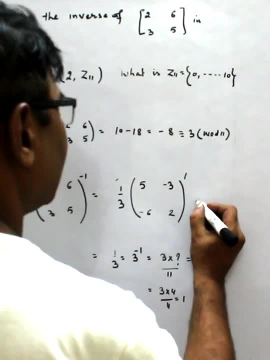 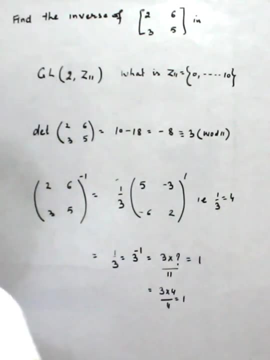 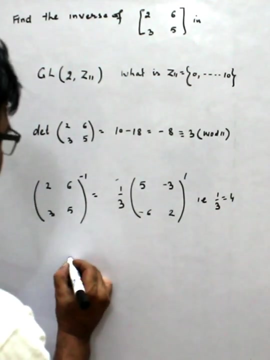 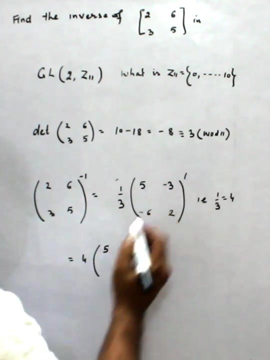 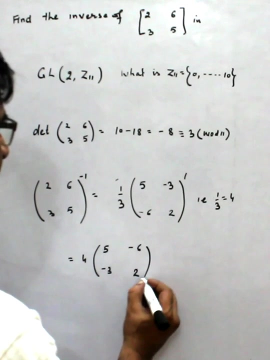 that mean I can write. I can write: 1 by 3 is equal to 4, 1 by 3 is equal to 4. now I rub this and then we move ahead. that mean this become 4 into 5. now I clear the transpose 5 minus 3 and this become minus 6 and this remain 2 as it is. 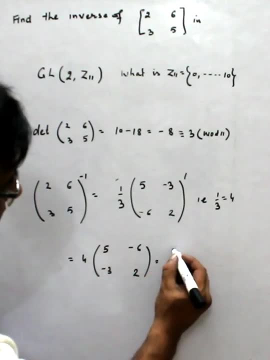 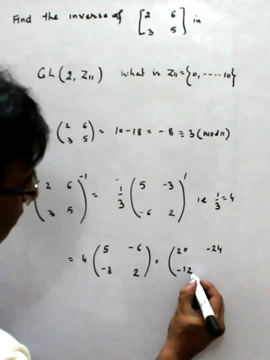 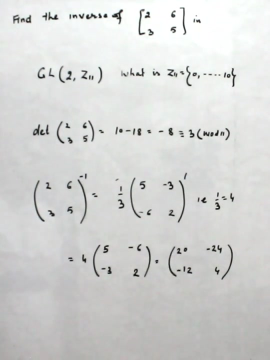 therefore, now I multiply 4, I take inside this number become 20, this become minus 24, this become minus 12 and this become simply 4. now 20 easily can be calculated. what become 20? 20 become minus 12 and this become simply 4. now 20 easily can be calculated. what become 20? 20 become? 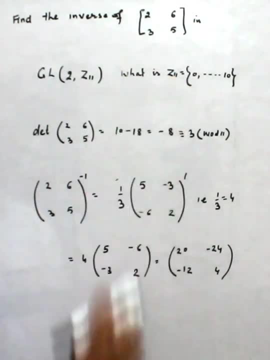 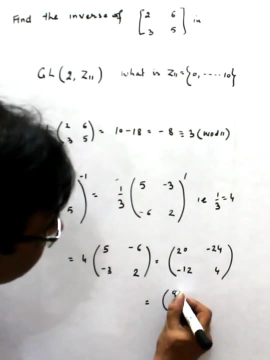 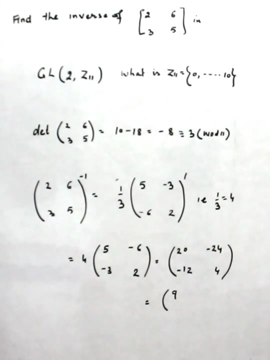 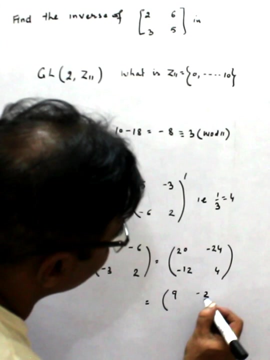 9. when I divide by 11, because we have the addition modulo 11, then this number equal to 9. now this: if I divide this become equal to minus 2 and minus 2 again. I can say: if I divide, this become minus 2 and this become minus 1 and this become 4. 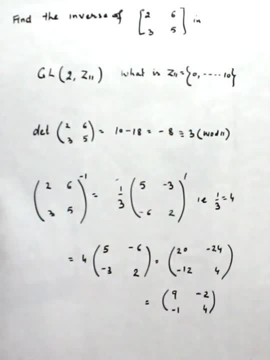 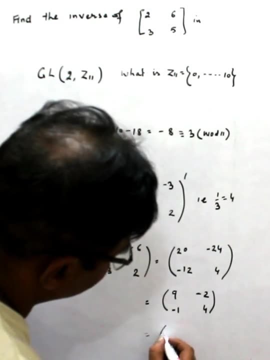 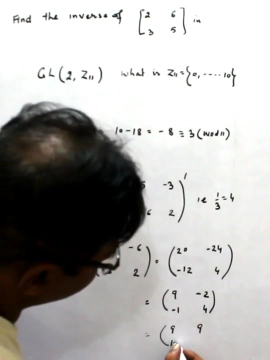 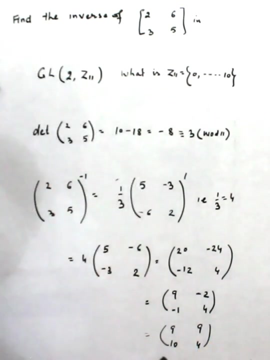 now this negative number. again we find the congruent number regarding minus 2 and minus 1. so this, simply: if I add 11, then this is 9. if I add 11, this become 9, and here this become 10 and this become this remain 4. so this is, this is. 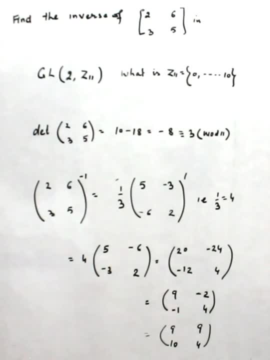 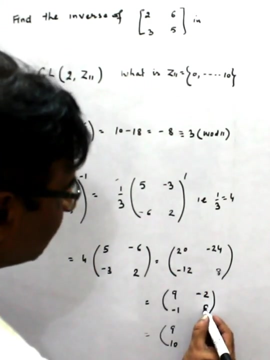 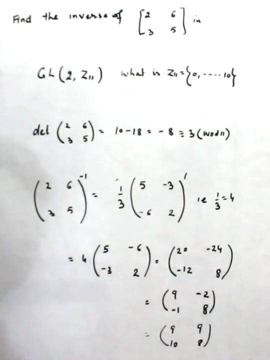 the inverse. this is the inverse of this matrix. sorry, one mistake, I think we have done this. 4 when multiplied this become 8, so it is everywhere 8. it is everywhere 8. so this is the inverse of this matrix. now we check if we multiply this with: 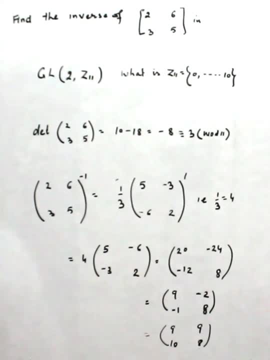 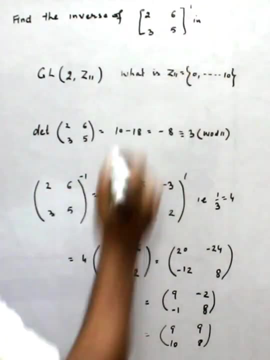 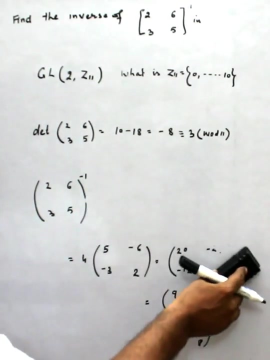 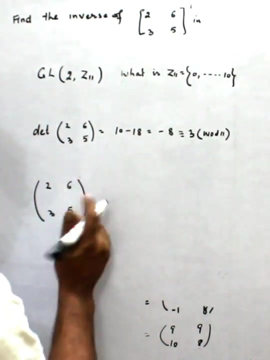 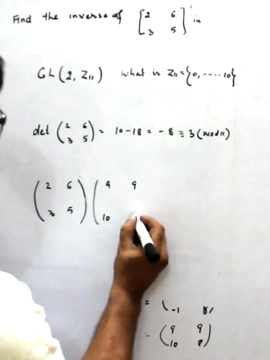 this. we should get the identity right. right, so it is. we are talking of the multiplicative inverse, that is minus 1, right? so we multiply this matrix, right, we can get the result to check whether our finding is good or not. so I multiply 9, 9, 10, 8. what I get now? simply this become: